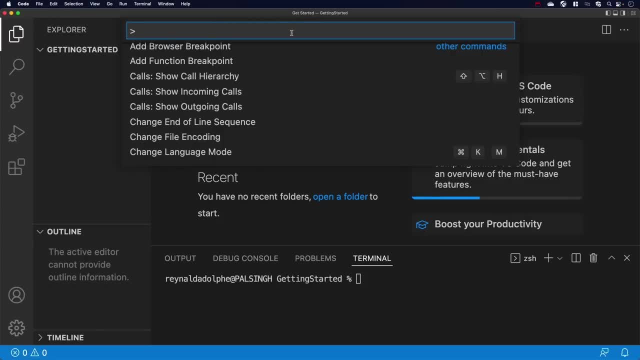 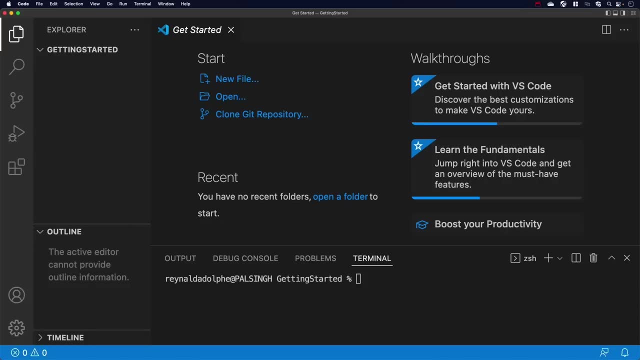 first option or use the shortcut. The command palette is very important as it is the control center for all commands in Visual Studio Code. At the bottom of the screen is the status bar, where on the left we'll see a number of errors or warnings and on the right, the current line. 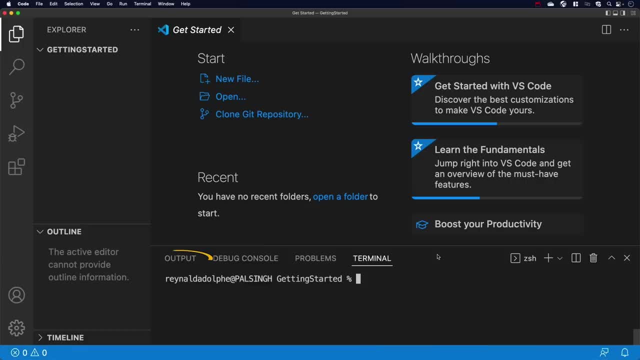 number and programming language. Right above that is the status bar, where on the left we'll see a number of errors or warnings and on the right the current line number and programming language, And above that is a panel for output or debug information, problem details and an integrated 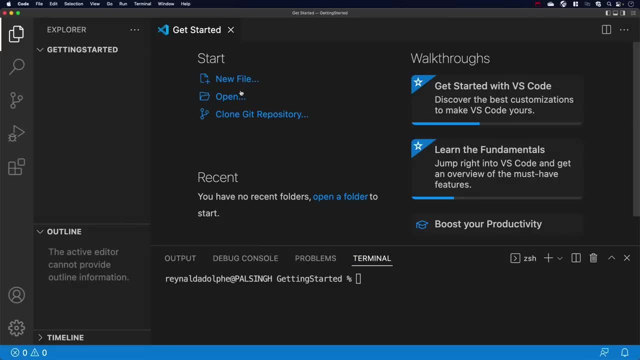 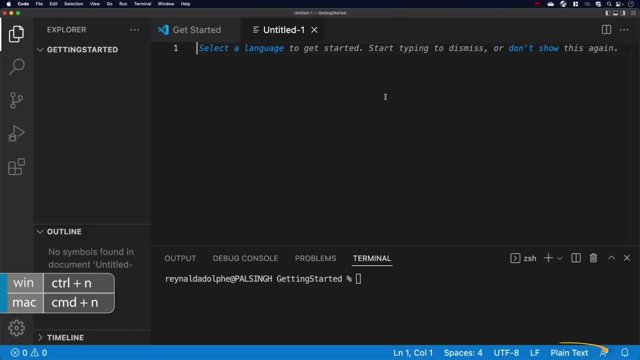 terminal. So let's go ahead and create a new file. I can go over here and select new file or hit command end And quickly notice at the bottom right-hand corner it says plain text. But once I start typing consolelog, open parentheses, immediately it notices it's JavaScript And at 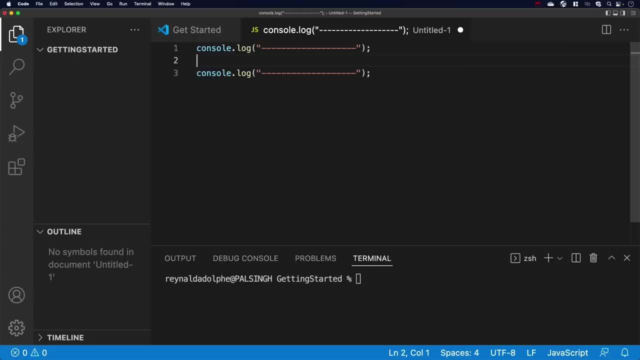 this point: once I start writing anything, I'm going to be able to see that it's JavaScript, And once I start typing anything else, IntelliSense is going to kick in. I write C-O-N and it's like: oh, you want to write, confirm console. It's trying to predict exactly what I want to write. I hit the. 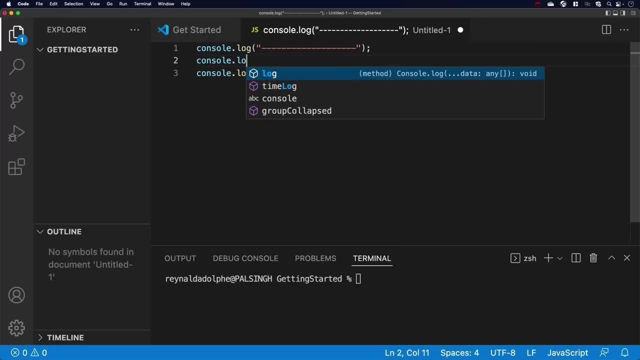 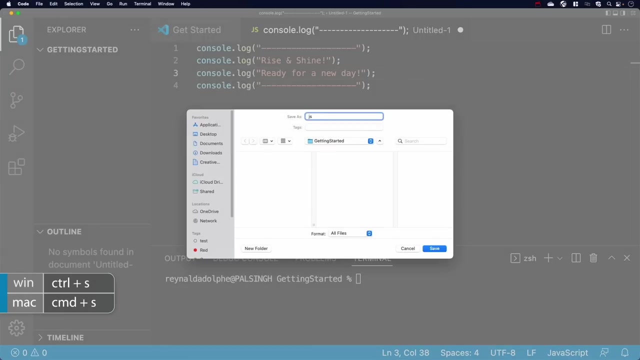 dot the letter L. Do you want to write log? Yeah, it's reading my mind practically. This is IntelliSense, It's that smart completion. All I'll write is rise and shine And, on the next line, ready for a new day. And if I hit command S, I will save my file as JS sample. 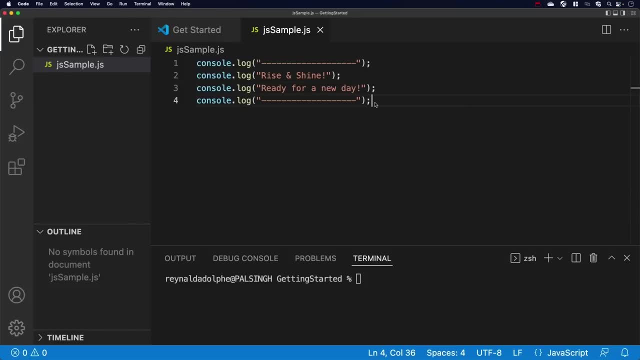 And hit save And you know you need to save whenever there's a change made. because if I hit the space bar here, you'll see that there's a dot that shows up which means I need to save. And if I want to have to avoid having to save every single time, I can go to file auto save and any 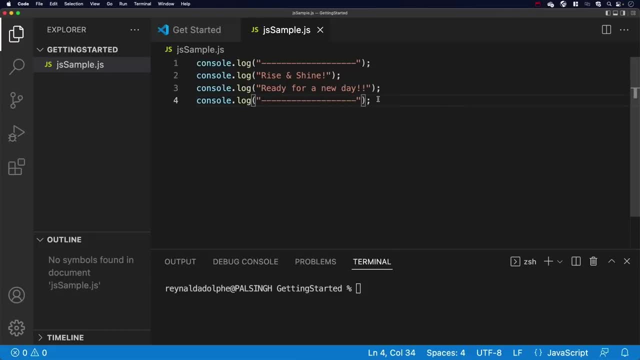 little change that I make, it immediately saves it. And now to execute our code, I hit F5.. And, as you can see below, rise and shine, ready for a new day. Now let's write something in Python. I'll create a new file. 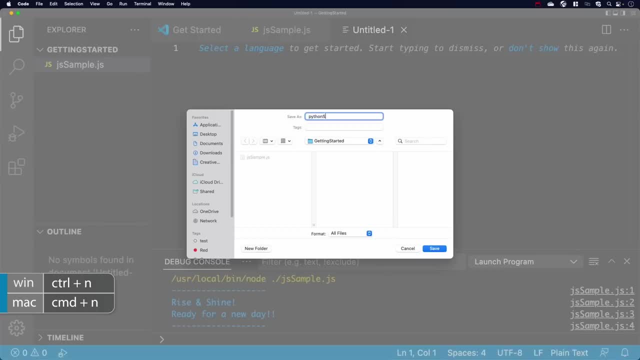 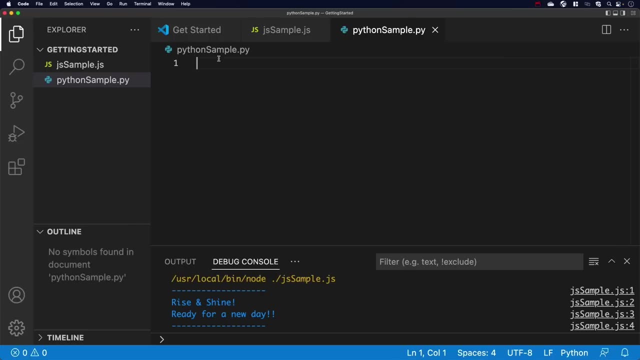 I'll hit command N and I will save it as pythonsamplepy. So Visual Studio Code at the bottom right-hand corner notices that it's Python. But if I start actually writing code you'll notice that I don't have that IntelliSense And in fact I could write almost anything here and it's not. 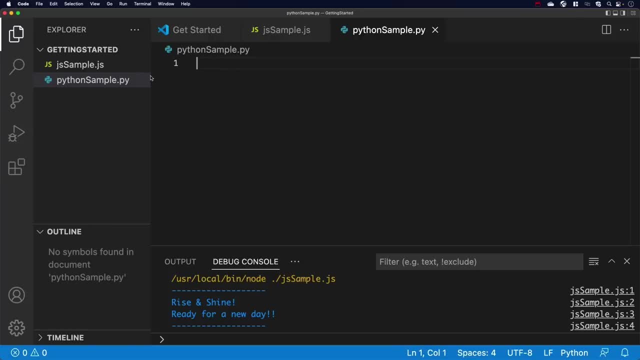 giving me any type of warning. So for a language like Python, extra support is needed, And that's where we could use an extension, which is the first one recommended here. So now we're going to go ahead and create our code, And we're going to go ahead and create our code And we're going to 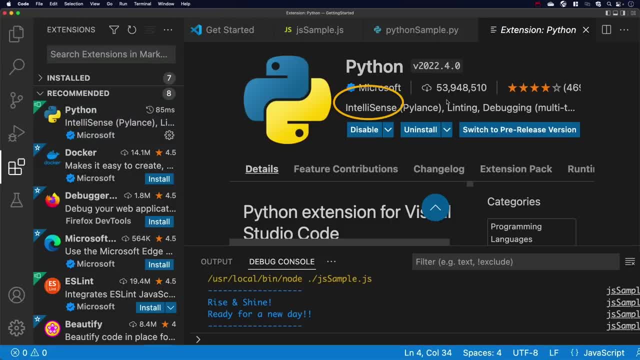 go ahead and create our code, And we're going to create our code And we're going to install it. And if you click on this little button here, it's going to show us the code that we're going to write into Python. And now it's installed And it will give us IntelliSense linting, which is 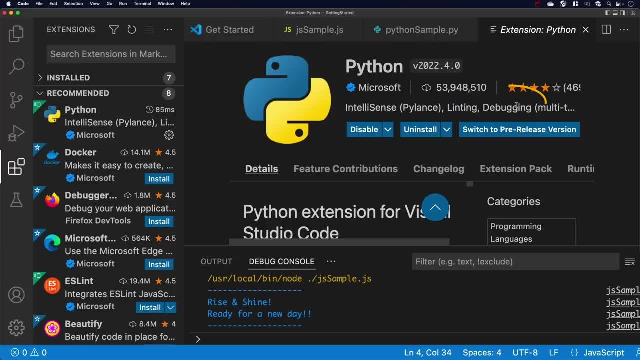 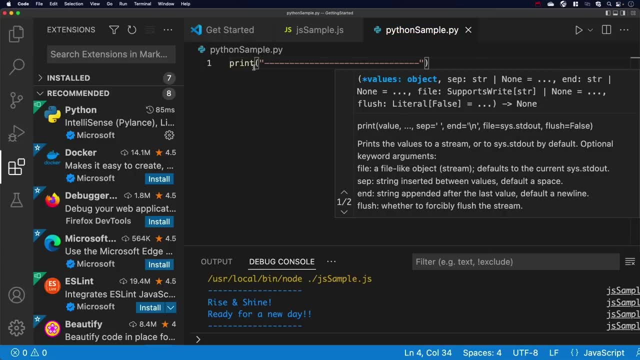 going to give us that squiggly line whenever there's like an error, debugging and some more capabilities. So now, if I start writing, I get that IntelliSense and I can finish writing my statement. And if I put in some nonsense here, it will give me a warning And now I can add some. 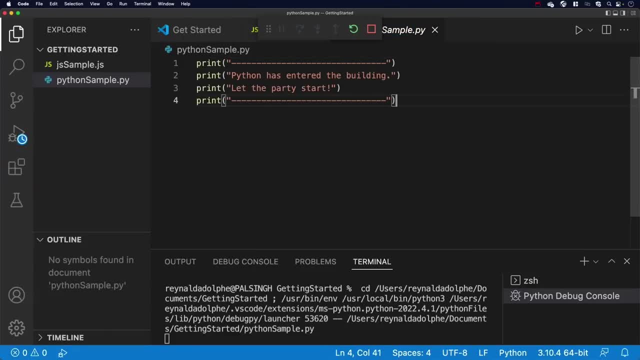 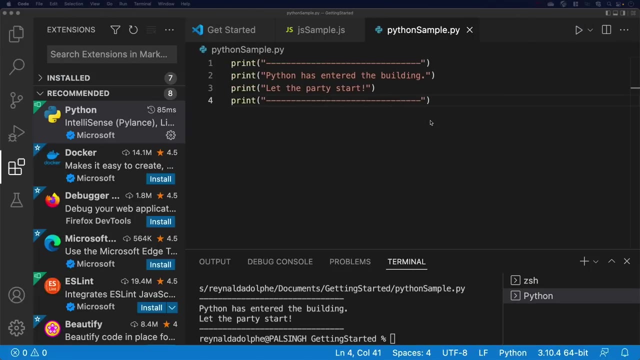 more code to execute it by hitting F5.. Python has entered the building, Or I could also enter the. execute it by hitting this run button here. now, how about demonstrating something with HTML? so, instead of creating a new file, what I do want to demonstrate is that you can just bring in a file into the Explorer section. so 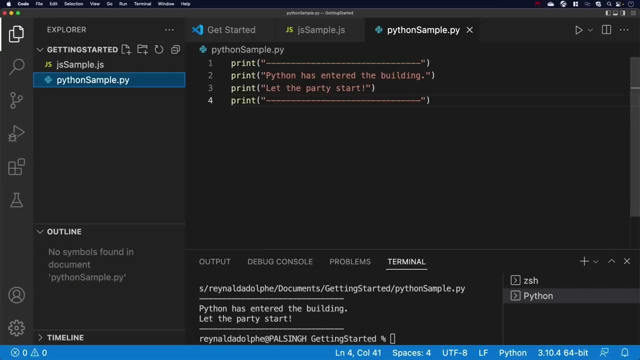 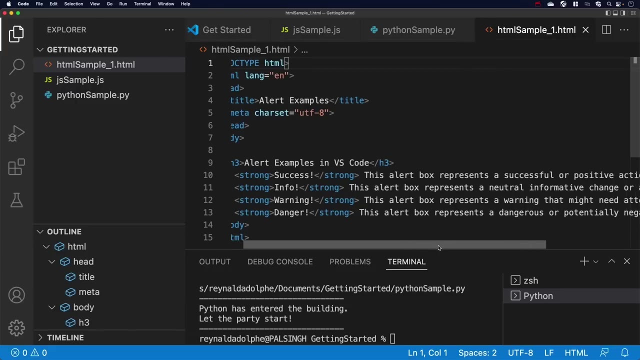 if I go and choose Explorer, I already have some prepared HTML that I'm gonna drag in from another folder, and when I drop it, a copy of this file will be created into my workspace under getting started. and here is just some simple HTML. now, with HTML, we can't execute it from the terminal, but what we can do is: 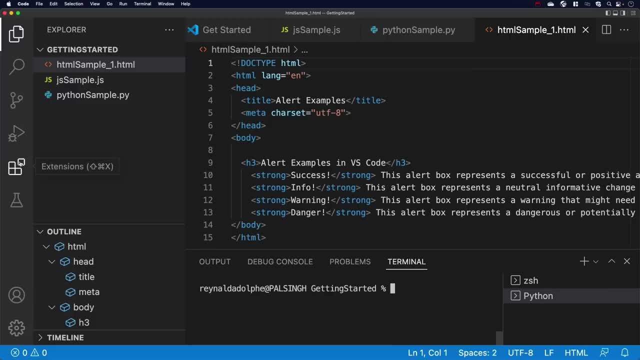 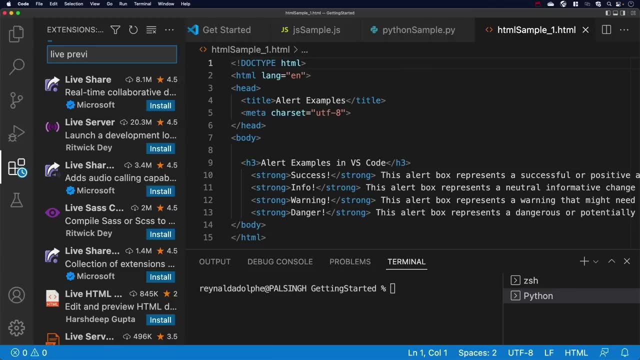 use an extension that will open a browser preview right in Visual Studio code next to your HTML and CSS. that extension is called live preview and we want the one specifically. by the way, that's the one that I'm going to use, Microsoft, which is the first one here, so I'll install that. head back to the 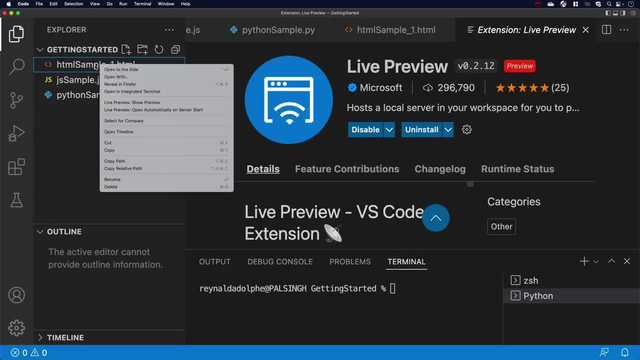 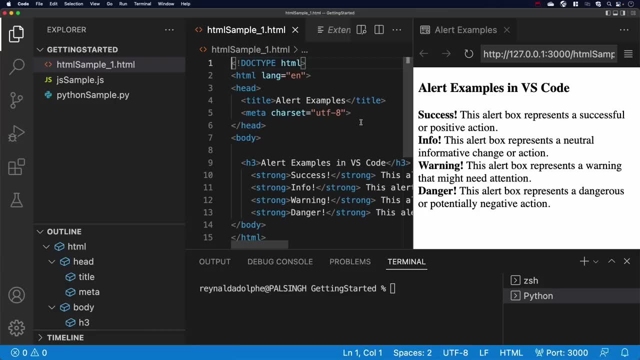 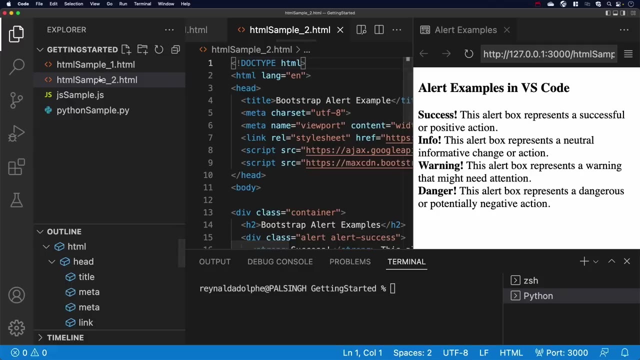 Explorer, and now all I need to do is right-click on my HTML file, select show preview, and there you have it within Visual Studio code. now, this version doesn't seem too attractive because there's no styling to it. I do have another example I can go ahead and drop in, and this includes some bootstrap. 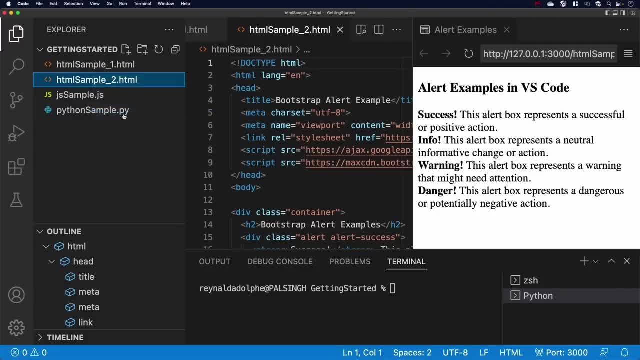 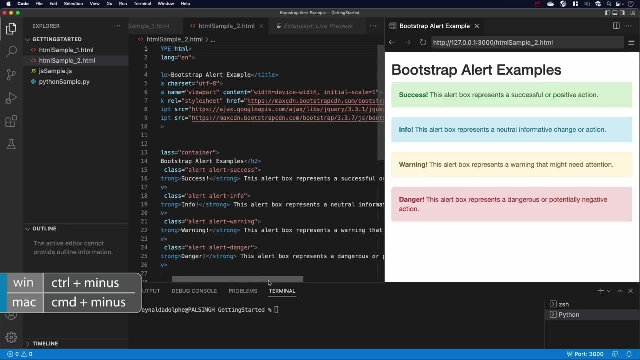 styling, and I'll do the same right-click show preview. this looks a little bit better. I'll hit command minus so you can have a better view, and what's great about this is you can make some changes and you'll see the results on the fly, and that is.